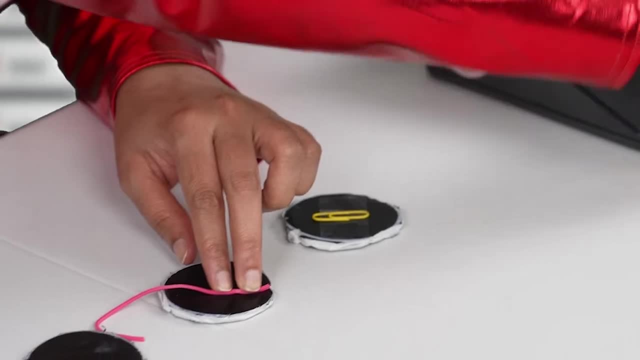 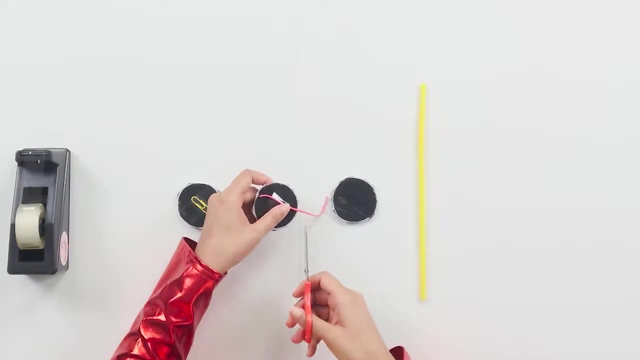 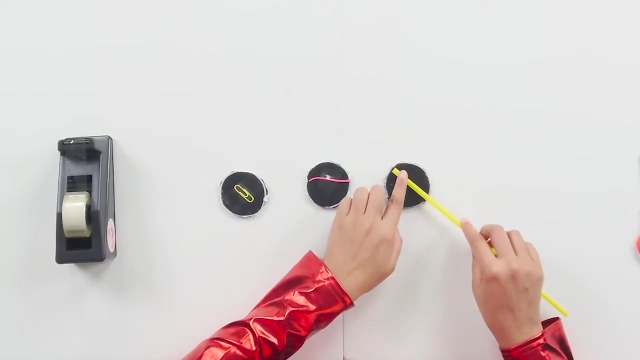 straight line. So grab some tape, stick the rubber band to the circle, and then you'll grab your scissors, because we will trim the rubber band so that it just fits within the circle. Okay, next we'll do the same thing with our straw. Bring the straw down to your 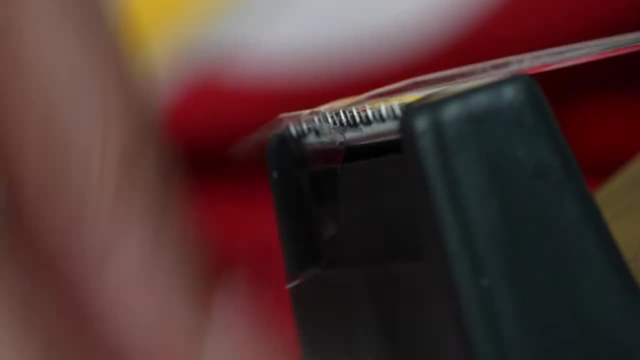 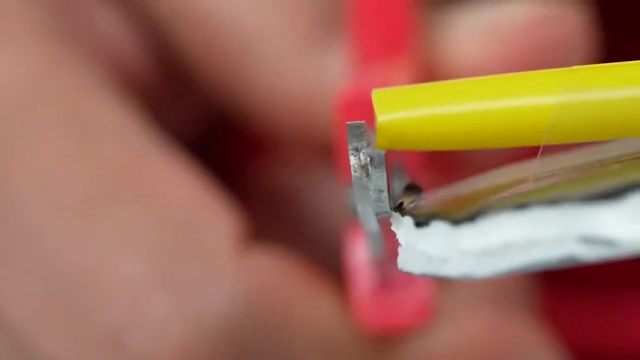 circle right to the edge. grab some tape, stick it down to your circle. grab your scissors and cut the straw so that it just fits within your circle circle Right. so next, let's fill a shallow bowl halfway with water. That looks pretty. 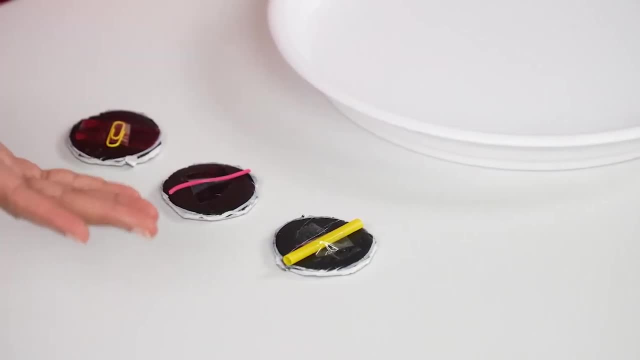 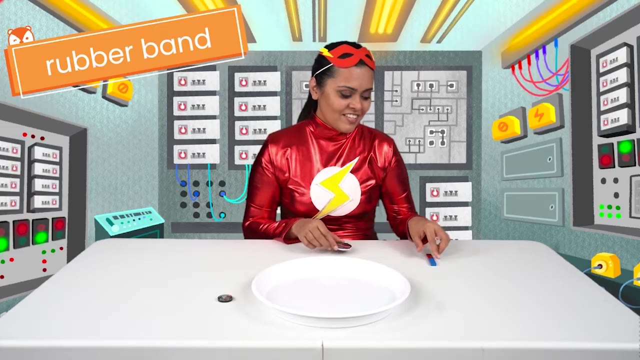 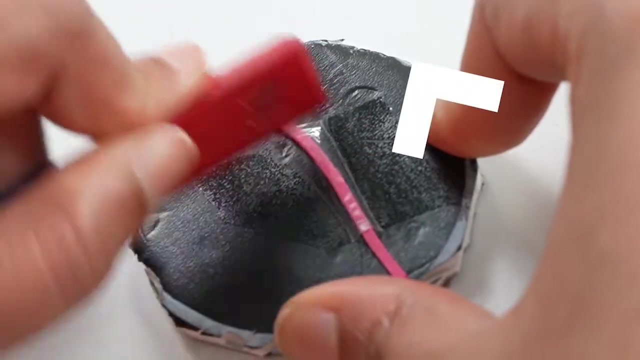 good to me. Oh, these three items actually kind of look like compasses, don't they? But which ones will actually work like a compass? So first let's magnetize the rubber band with our magnet rubbing it in one direction. So let's rub this for 30 seconds, Next we're. 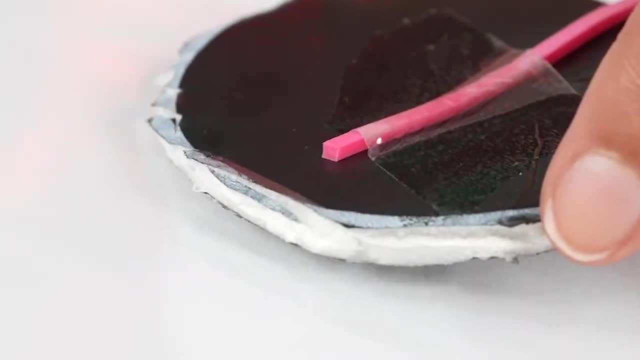 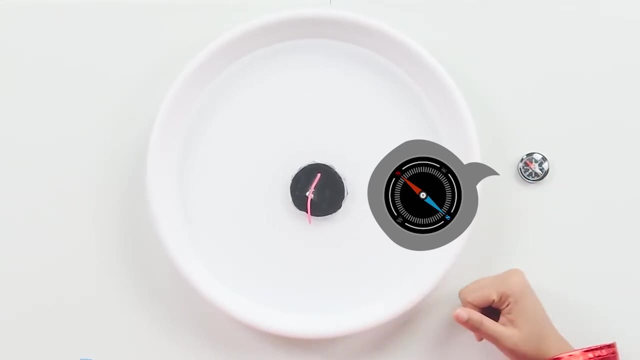 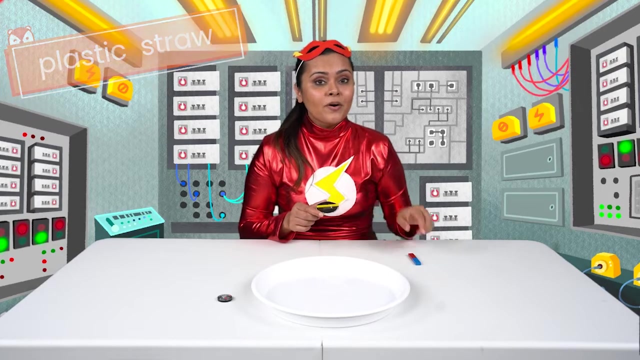 going to place the rubber band into the water. observe your compass and let's see if it turns and acts like a compass and faces north. It doesn't seem to be turning around. It's still facing in a different direction to the compass. Next we're going to go ahead and 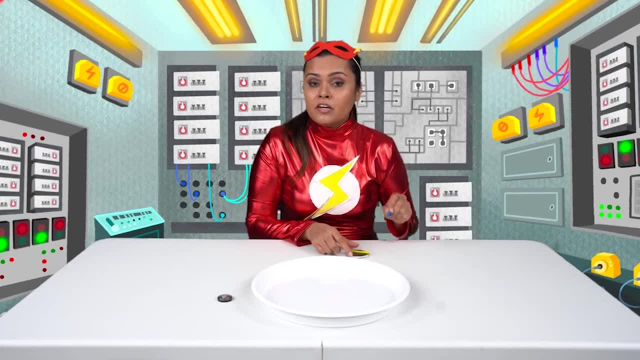 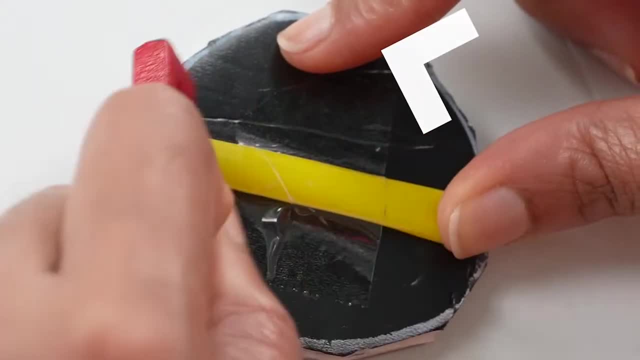 magnetize the plastic straw by rubbing the magnet over it. But remember you have to stroke it in one direction, because if you do it both ways, the experiment won't really work. We have to do it for 30 seconds. So next we're going to take our magnetized plastic straw and place it lightly on the 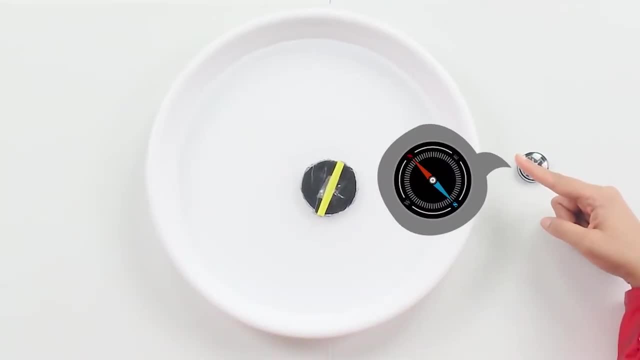 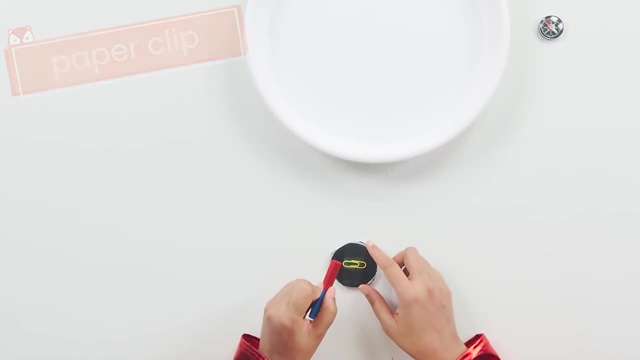 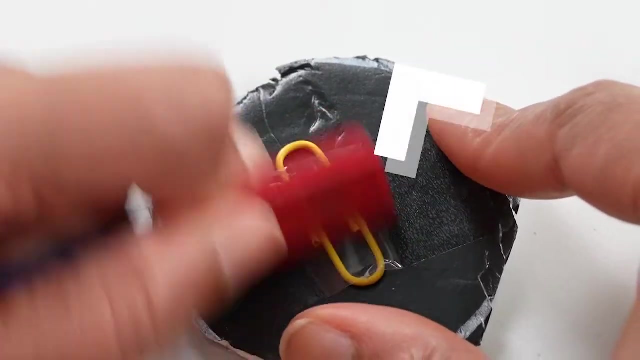 water Doesn't seem to have turned at all. It's still in that direction. Alright, let's magnetize the paperclip by rubbing the magnet for about 30 seconds, and remember we need to rub it in one direction, not both ways, otherwise the experiment won't work. We're. 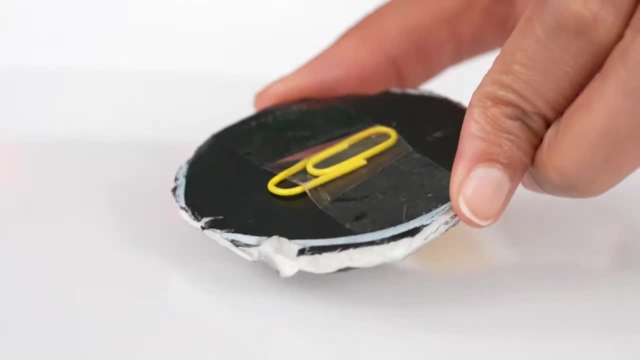 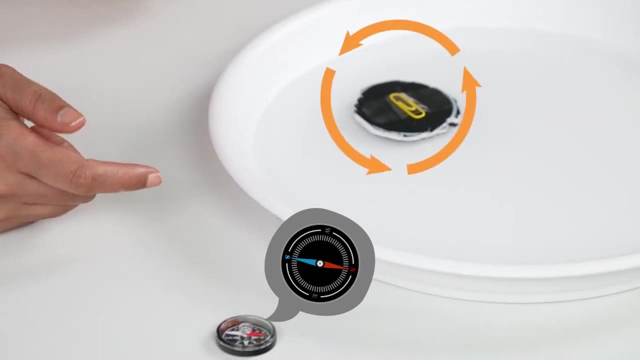 going to place our paperclip into the water lightly and watch the direction of the needle of the compass and put it in in a different direction of the needle. Oh, it seems to be spinning a little bit. If it's magnetized it'll follow the same direction of our compass. 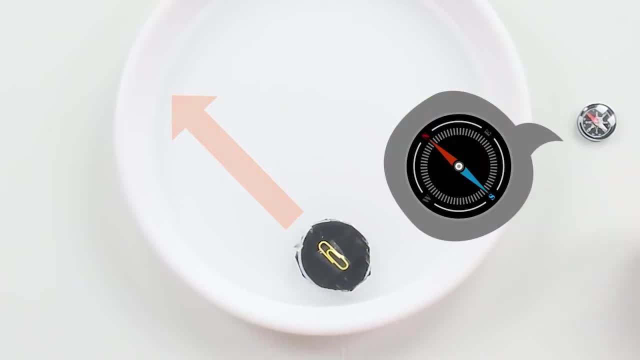 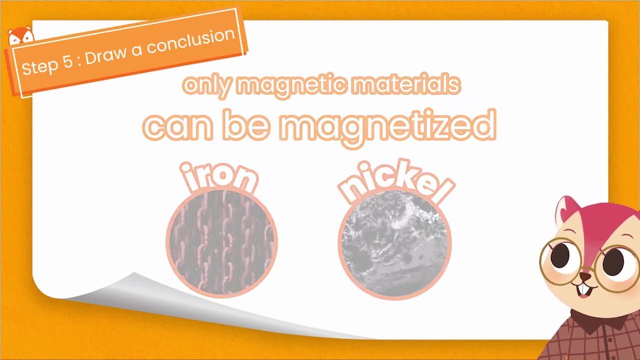 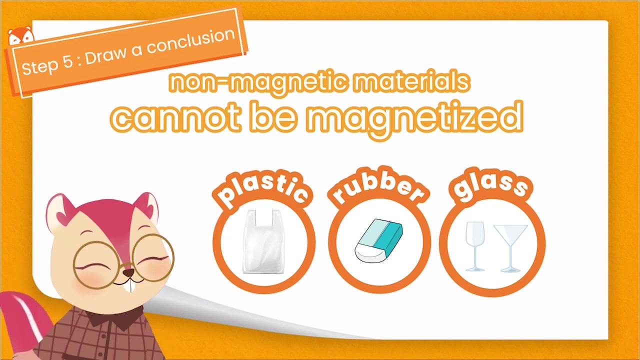 And it stopped right there, in the same direction of our compass. Wow, Only magnetic materials like iron and nickel metal can be magnetized, whereas non-magnetic materials like rubber, plastic or glass cannot be magnetized. Want to watch the full video?